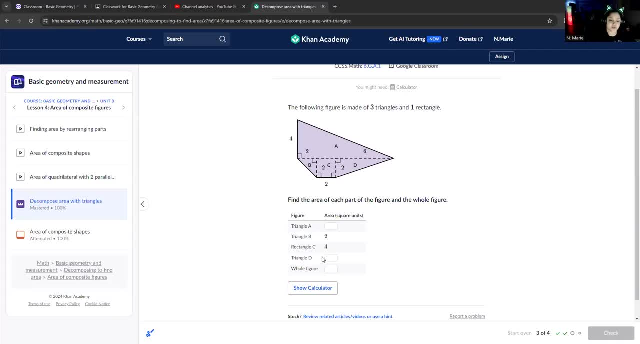 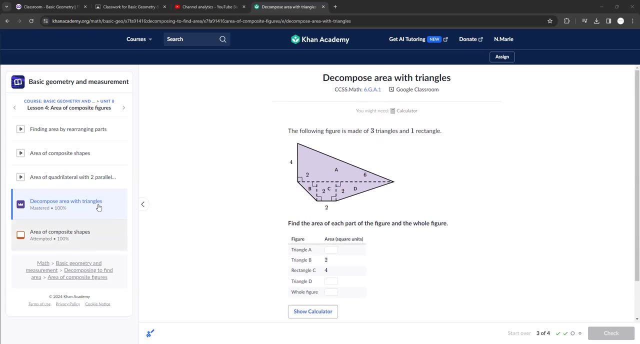 Welcome. So we are on part two of this unit, which is decomposing to find area, And so now we're doing it with triangles and area of composite shapes. So the first part kind of sets you up for the second part, because they split it up for you And we already know how to. 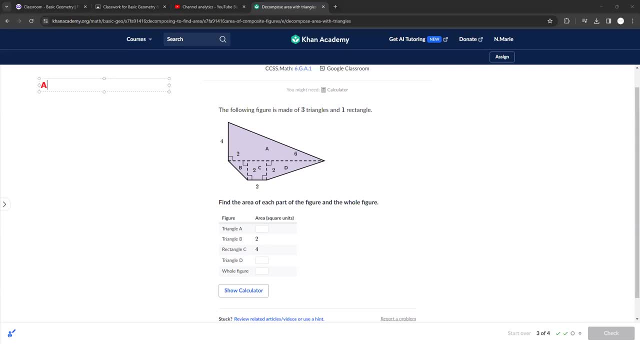 find area of rectangles and squares. I hope So. area for rectangles and squares is basically length times width, or side times side, And for parallelograms we know it was base times height. I'm just going to put rectangle And then there's no parallelogram. So then area of triangles. 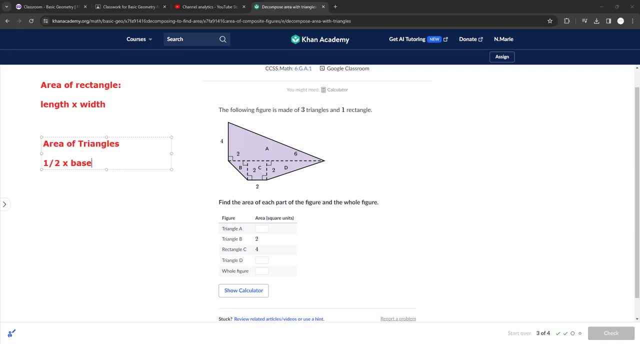 would be one half times base times height, or base times height divided by two, whatever you want to do. Okay, so this helps you prepare. So make sure you pay attention to each step. So for triangle A, they want you to find the area. 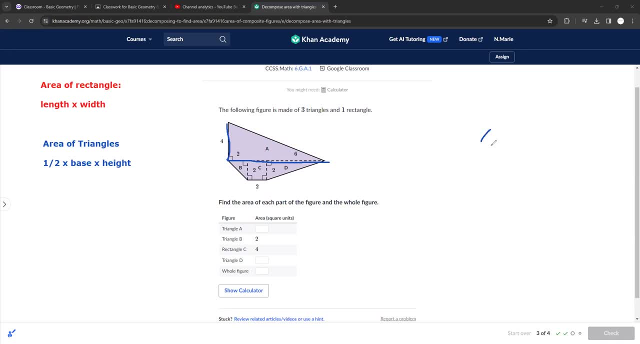 The area would be the base times the height. The height is four. The base is a little tricky So you have to like fill in the blanks. This is two, that's two and that's six, So then that would be six, seven, eight, nine, 10.. So that would be four times 10 divided by two, which is 40 divided by. 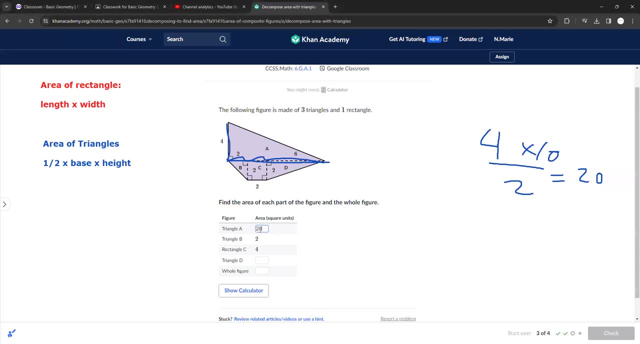 two, which is 20.. So the area for triangle A is 20.. They found the area for angle B, which is 40. But make sure you do it, just so you know how to do it on your own if you had to. So this is two. 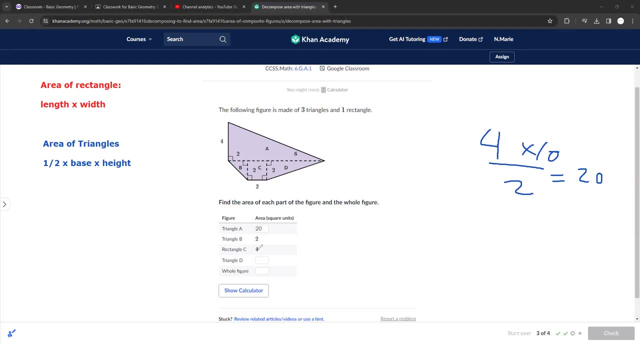 times two, which is four. Four divided by two is two. For rectangle C, length times width, which is four, That's what they put. And then for this rectangle here we would do: base times height, divided by two, which is six, times two, which is 12, divided by two, which is six. And now we want: 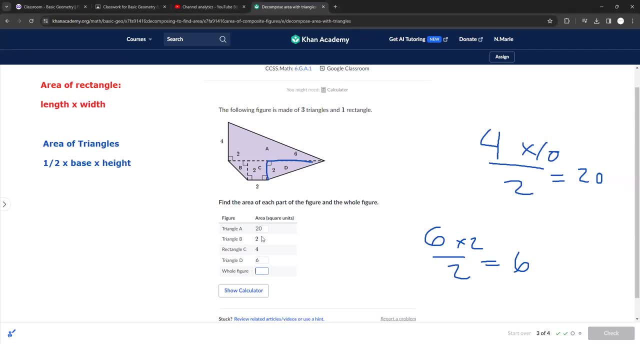 to add all of this up. So this is 10, that's 20.. So that's 30, and then two, And so this is help. Like I said, it's helping you set it up if, in case, you were to do it on your. 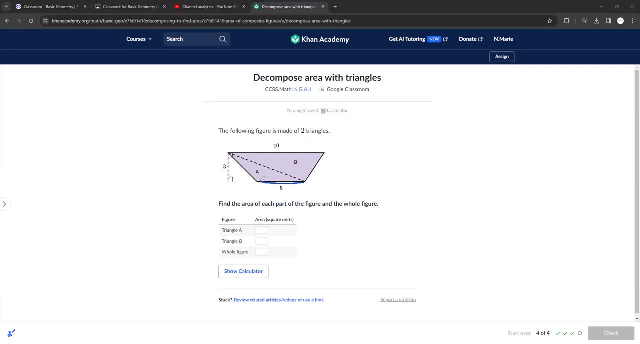 own. So triangle A, so remember it's base times height. So that would be five times three divided by two, which is seven, 7.5.. So for B, what's the base for this one? Triangle B is 10 units and its base is three. That one's kind of tricky to do, because remember the base. 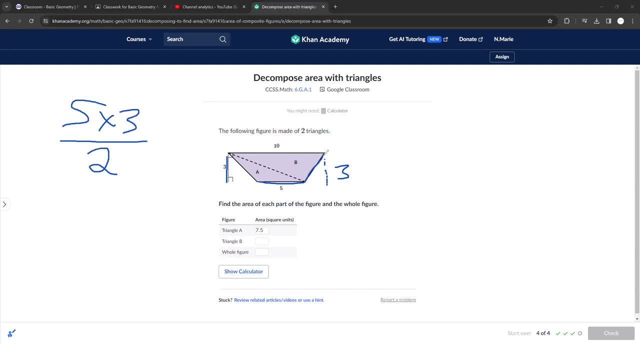 and higher perpendicular. So this is the wait. that actually would be the base. Hold on, Let's see for this one. Hmm, So you didn't give us the base for this. Let me think: Okay, So for sure, the height of that triangle, unless they saying, oh, they might want you to do this. 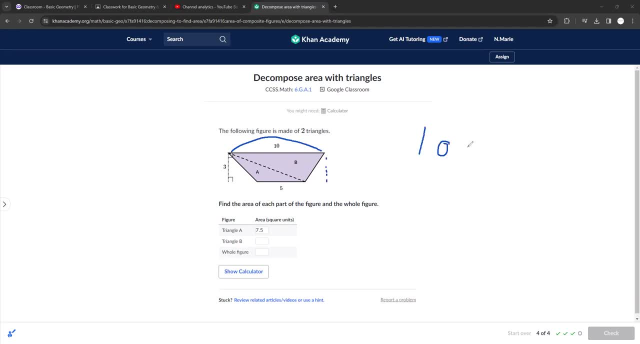 for base and this for height, and divide by two. Okay, So that would be: 10 times three equals 30 divided by two, which is 15.. And then we add these together and we get 22.5.. All right, So yeah. 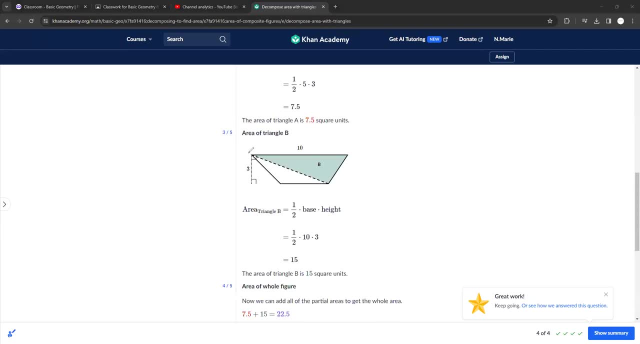 that one was a little tricky, cause I'm I was thinking too much into it. but for this triangle B, this I was thinking that This was like the triangle should face upward, like this Cause. remember, these are rotated, So you kind of have to identify what's the base and the height. but for this one, 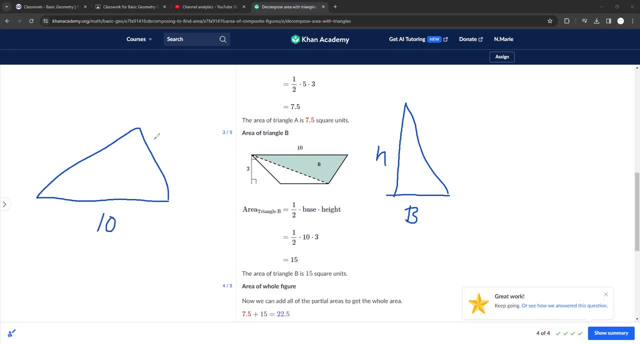 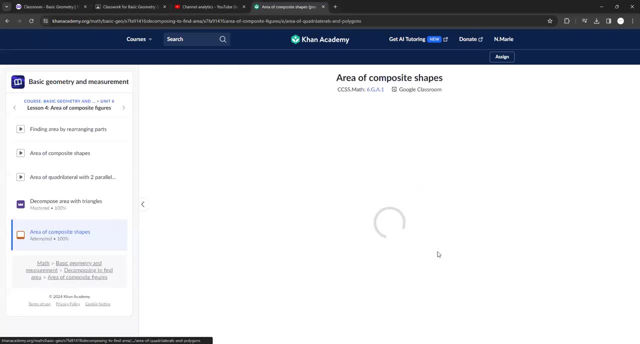 they actually wanted the triangle more. So facing this direction with this is the base and this is the height. So just careful with that. You kind of have to train your eye and geometry, Okay. So last part we're doing is area of composite shapes. So for these you need to. 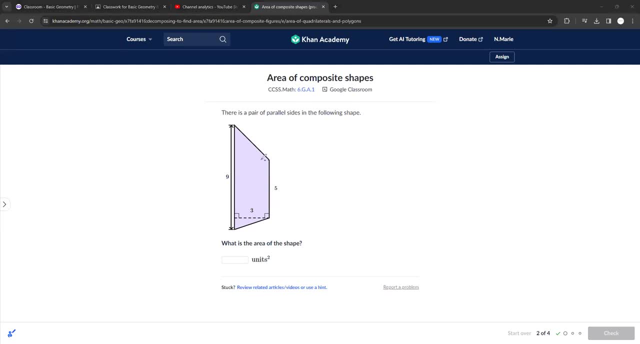 split them up on your own. So I'm going to split it into another triangle there. If that's five and that's three, Let's see We can also. Okay, So if I did it like that, if that's five, the entire thing is nine. 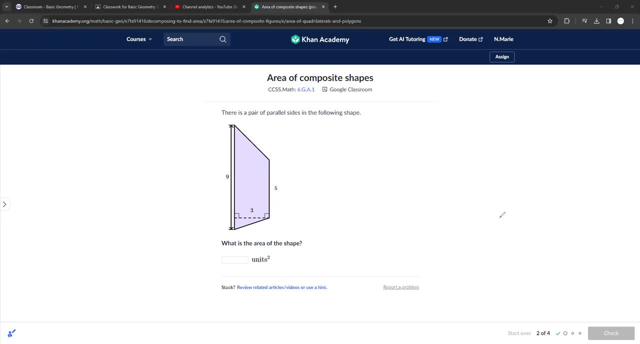 Hmm, Let's think on this one, All right. So these can be a tricky thing. I could find an area of a triangle. I could find an area of a triangle. I could find an area of a triangle, So I could do a trapezoid formula which would be base one plus base two. 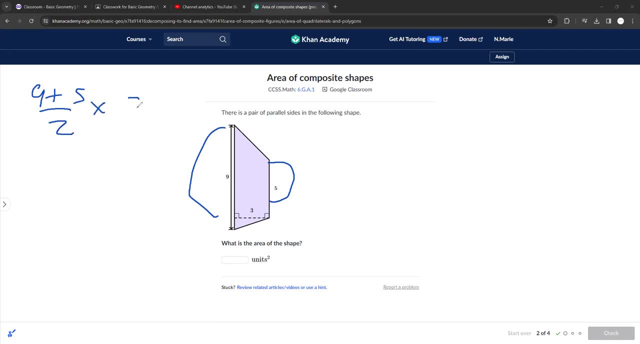 divided by two times the height. I could do that, but we're in a unit where you're not supposed to know trapezoids yet, I suppose, So let's do it the other way, Okay? So remember, you want to split these up, So spend some time looking at these and seeing. 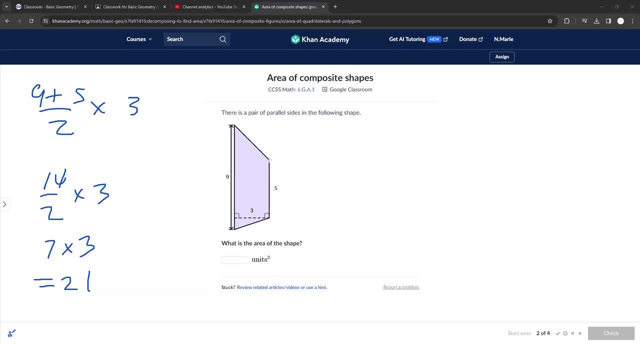 how you would split it up. So I would split it up like this. I was trying to think of a. yeah, i was thinking, looking at it different ways, but no, this would be better only because of the dimensions that they've given you, right. so they've given you. this is five and that's three. 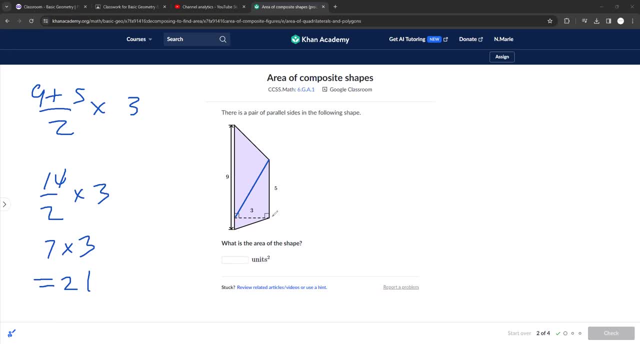 um, and so then you also have that little triangle there, okay, so if that this piece is nine, actually, hold on, let me split it differently. i wonder actually, let's look at this one. i want to see how they split this. but you can see, area of a trapezoid formula would work, but let's see how they split this actually. 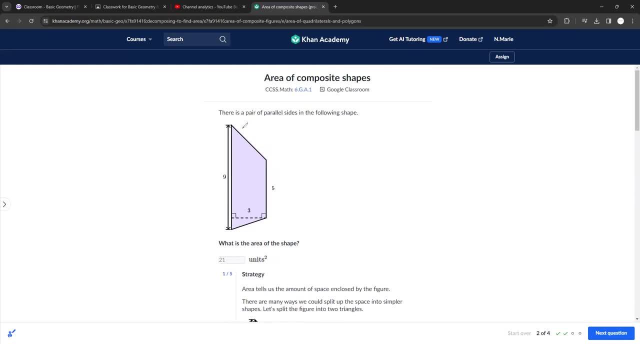 okay, so they split it like that that. so yeah, play around with it. sometimes the splitting it part is confusing. okay, so we would split it like this and then find the area of the two triangles. so this would be a base of five and then you would have this lado triangle. that would be the area. 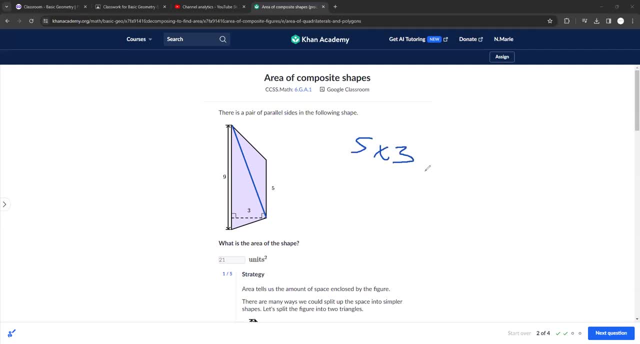 end of the triangle, which would be the base of the triangle, and then you would have the jedd people height of 3 divided by 2, which is 7.5. And this would be a base of 9 with a height of 3. 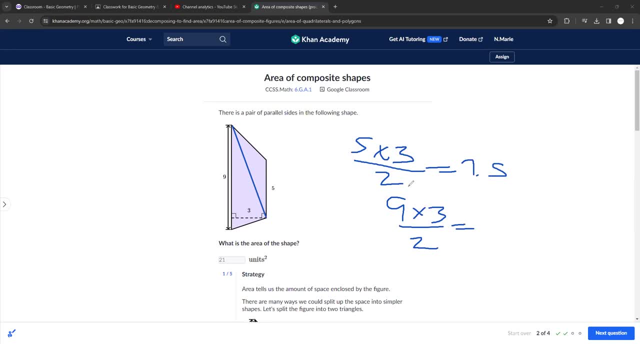 divided by 2, which is 9 times 3, is 27.. 27 divided by 2 is 13.5.. So if you added those together, you would get 21.. So spend some time practicing splitting these up. All right, so for this one. 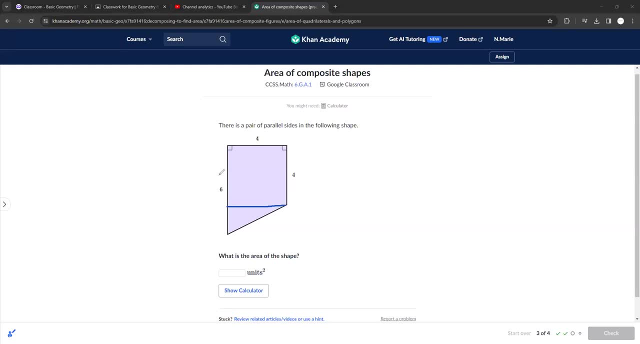 we could split it up like this: If that entire thing is 6, and that's 4,, this should be 4, then this is 2.. And then this is also 4.. 4 by 4, that square, there is 16.. And this: